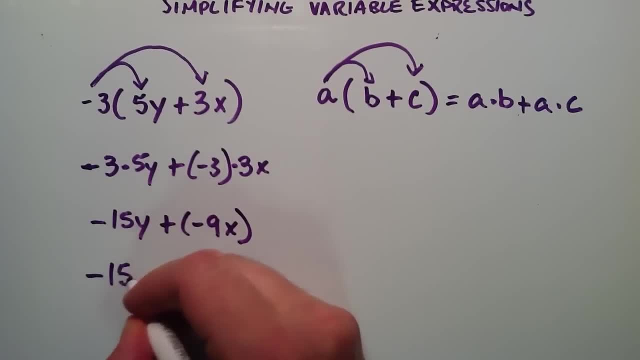 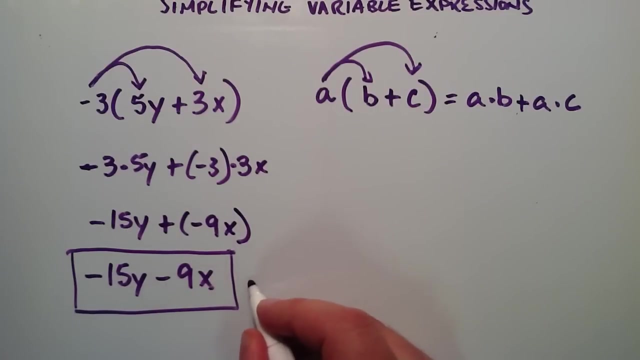 So we can rewrite this bottom part as negative 15y minus 9x, And so we've simplified, We've simplified this expression right here and it looks like this: So this is basically our answer, This is our simplified expression, And so this tells us that this is the same thing as if we were to write negative 3 times 5y plus 3x from above. 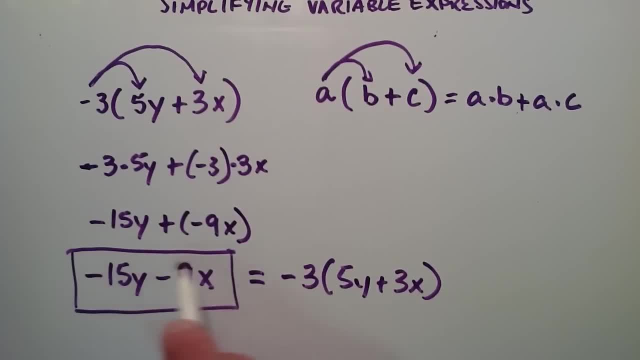 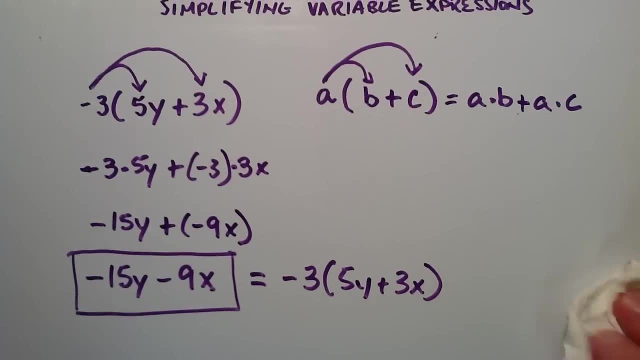 So these two are equivalent. This one is a little bit more simple. So that's how you simplify a variable expression using the distributive property. I'm going to go ahead and do one more example right now, And so we're just going to. 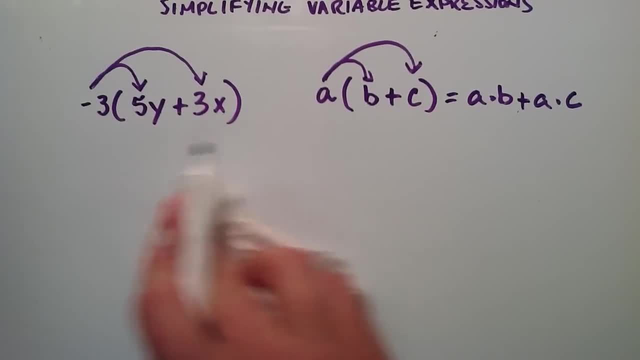 We're just going to basically extend the distributive property now. So up here I say that we can distribute a into two different terms. But it turns out with the distributive property that we can actually distribute a into as many terms as we need. 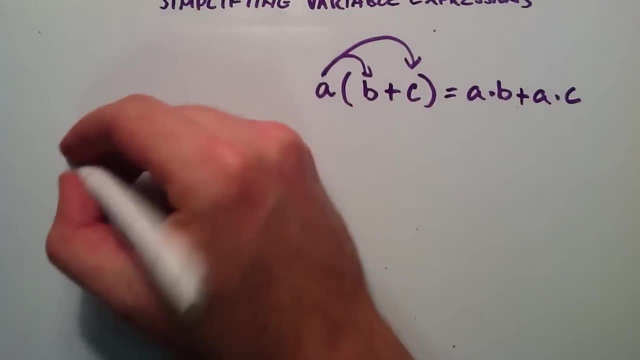 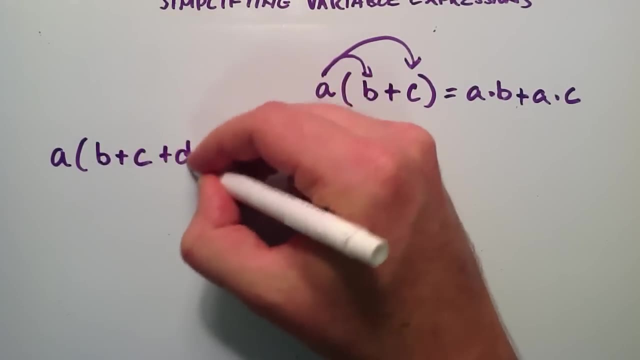 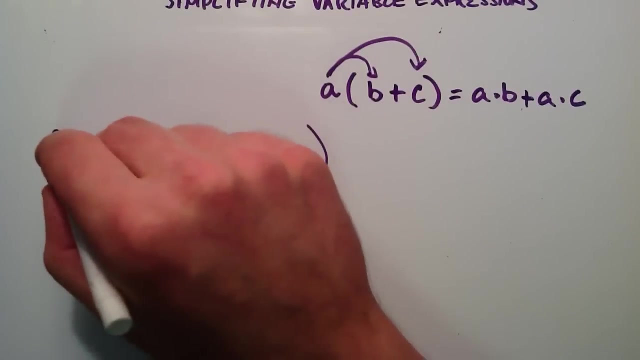 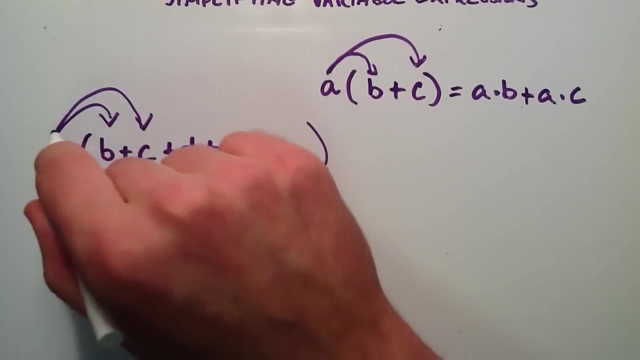 as long as they're all within the same grouping mechanism. So basically we have some number a and inside of the grouping we have, say, b plus c plus d plus as many different terms. So you can distribute a times b, a times c, so it would be a times b plus a times c plus a times d plus. 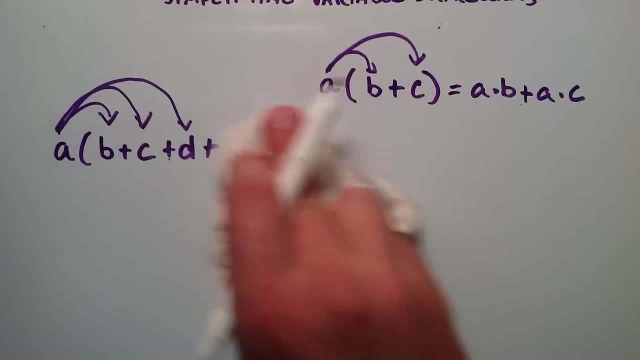 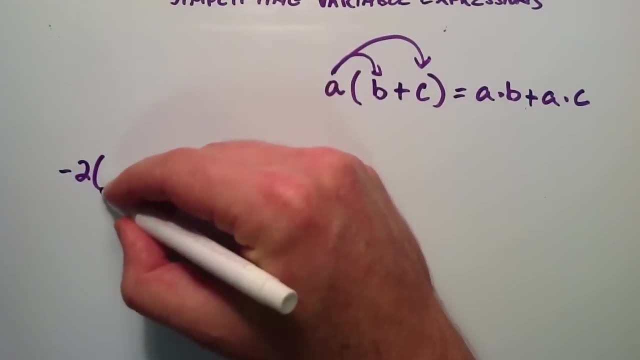 and you just keep that pattern going. So let's go ahead and do that. Let's do that with this next example here. Let's do negative 2, and we're going to do negative 2, and then inside the parentheses, we have 5x plus 3y. 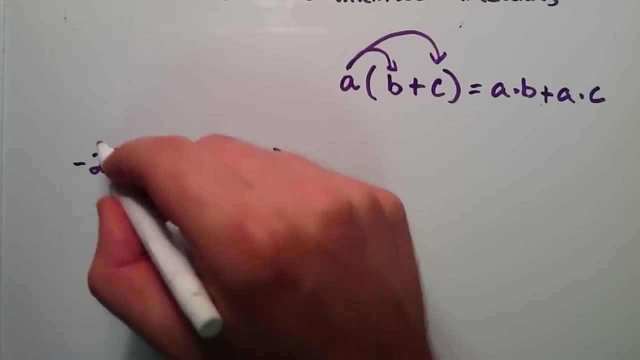 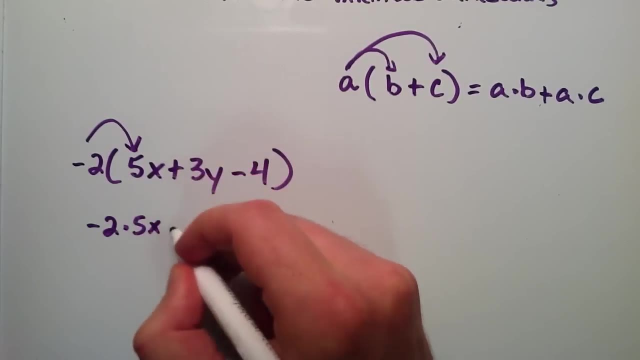 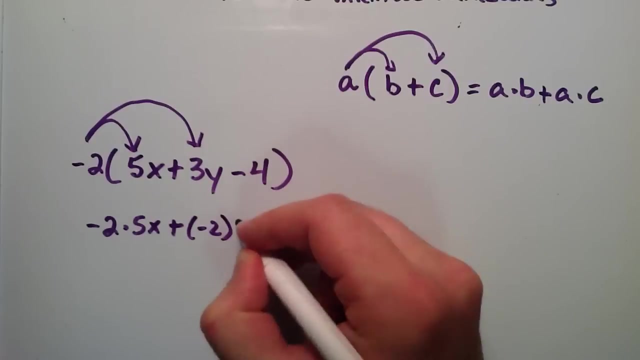 And so we're simply going to distribute this negative 2 into the first term. So this becomes negative 2 times 5x plus negative 2 times 3y. So this is negative 2 times 3y minus, So it doesn't actually have to be a plus like we have here. 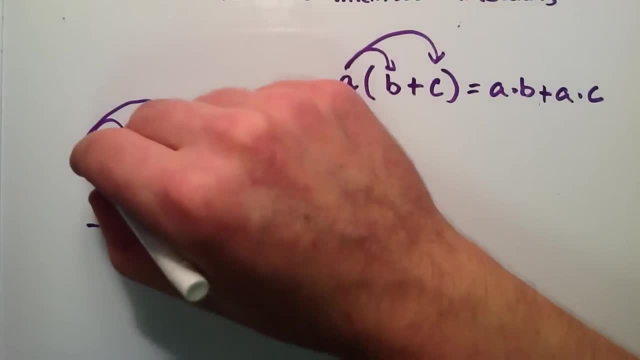 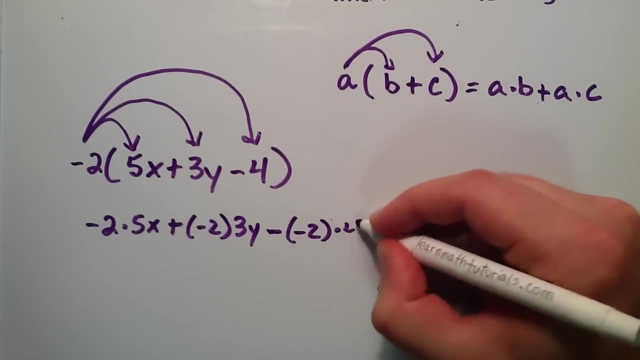 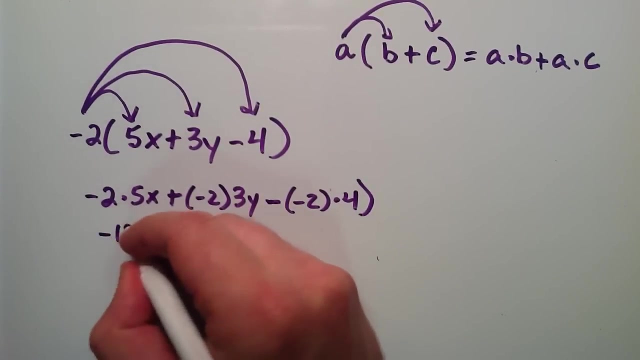 This time we're just going to go ahead and write the minus down And then we do a negative 2 times 4.. So this is negative 2 times 4.. So then we just simplify this right here. So a negative 2 times a positive 5 is a negative 10, and then we have the x.